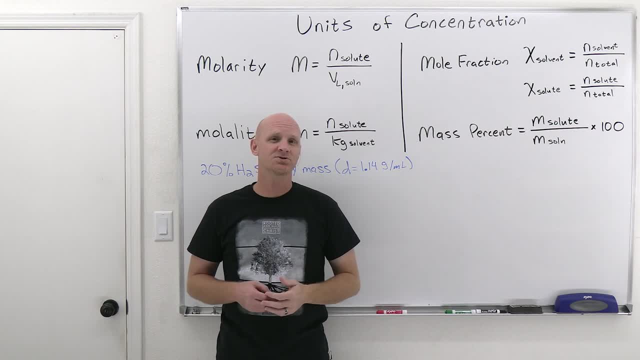 My name is Chad, and welcome to Chad's Prep, where my goal is to take the stress out of learning science. Now, in addition to college and high school prep, we also do MCAT, DAT and OAT prep as well. Now this lesson's part of my new general chemistry playlist. I'm 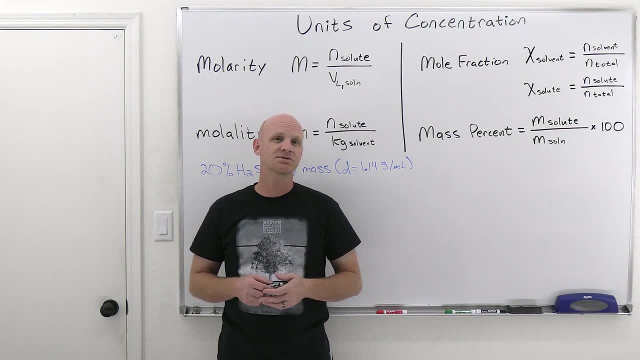 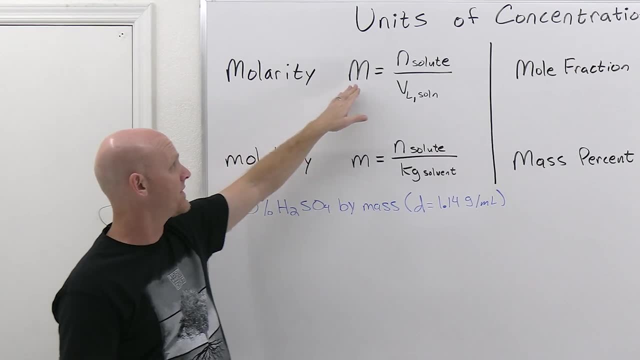 releasing several lessons a week throughout the school year. so if you want to be notified every time I post a new one, subscribe to the channel, click the bell notification. All right, so quick review here on what molarity is And molarity with a capital M here is 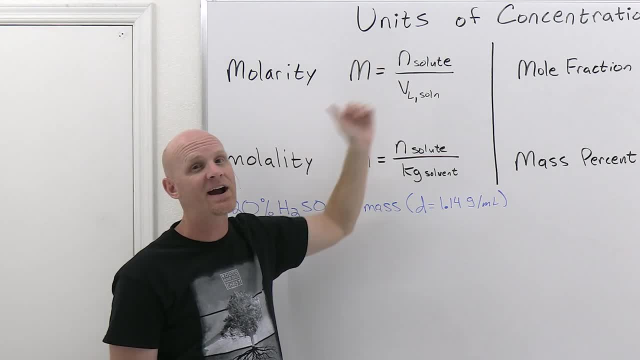 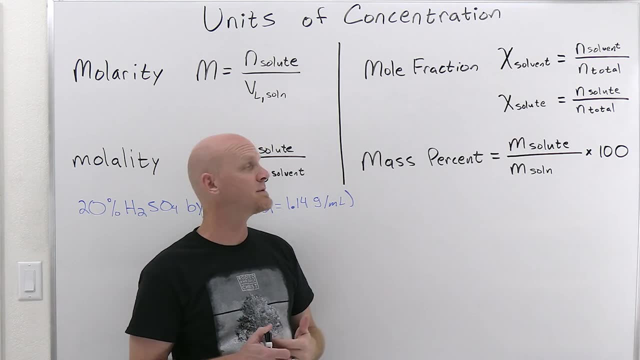 the moles of solute over the total volume in liters of the entire solution, And then mole fraction is just the fraction of the moles that are whatever you're talking about, And so in this case it actually becomes convenient to either look at it from the 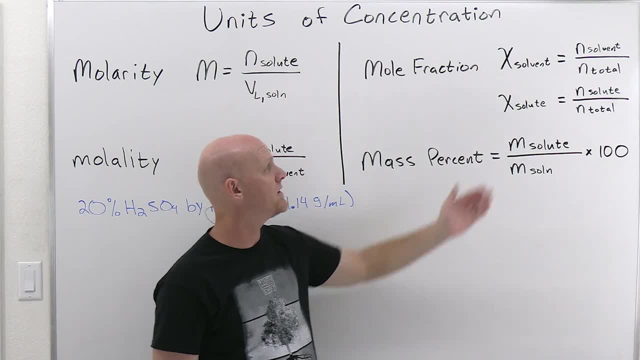 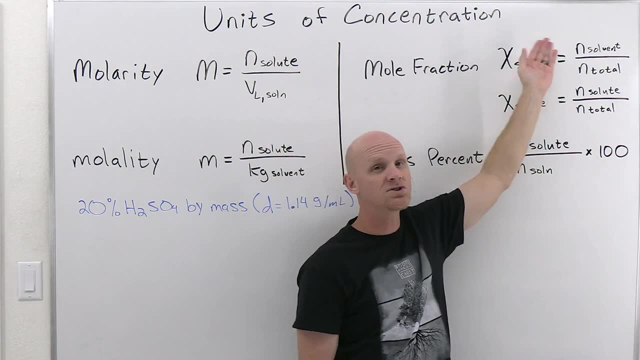 perspective of the solvent, which is one we will use in the next chapter, or from the perspective of the solute, potentially as well. And so if you're doing the mole fraction of the solvent, well then it would just be the moles of solvent over the total moles. 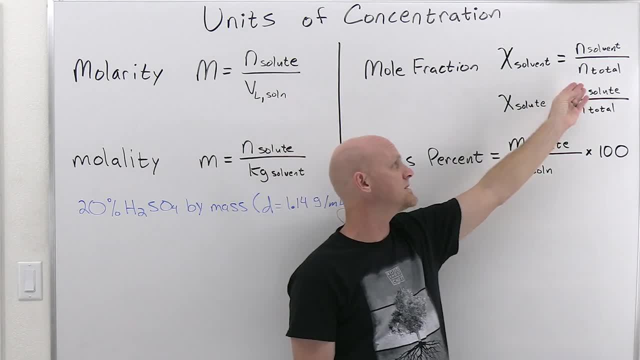 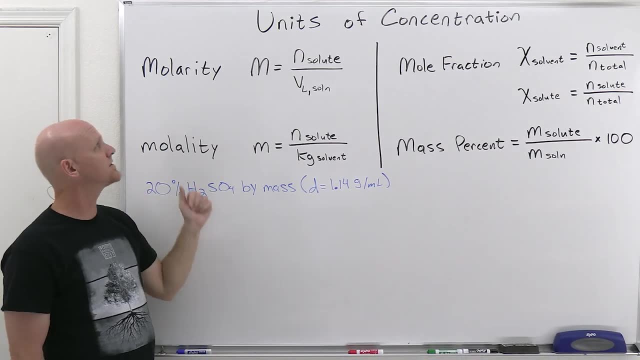 solute and solvent combined, Or, if you do the mole fraction of the solute, it would be the moles of solute over the total moles combined. All right, molality is next, And so students sometimes will confuse molarity and molality- obviously very similar names here, So molality. 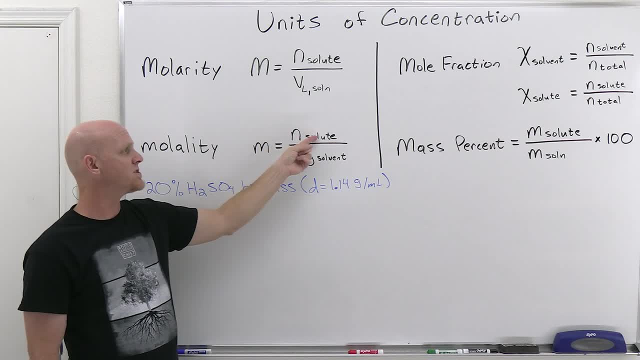 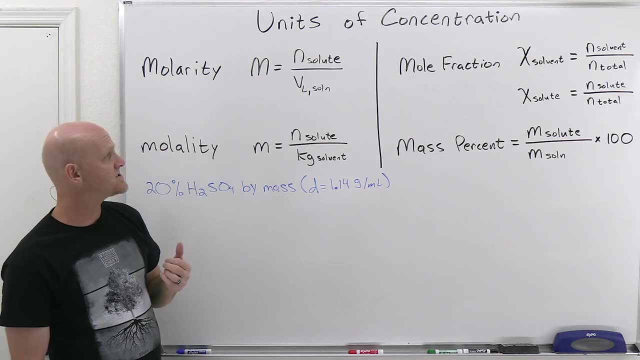 we use a little m to abbreviate here, and it's moles of solute. But instead of being over the total liters of solution, it is now over the kilograms of solvent, And this is an important distinction here. So as you add more and more solute to a solution, its volume does change. But as you add 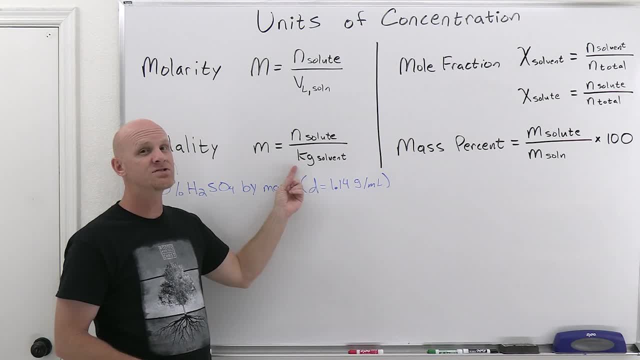 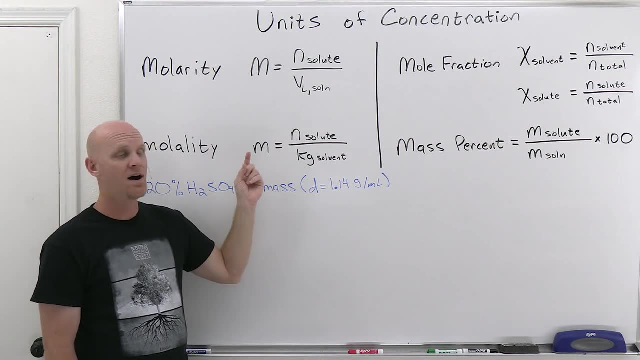 more and more solute only to a solution. the number of kilograms of solvent does not change, And so we'll definitely see some differences here, And it turns out for a couple of the colligative properties. this becomes a better reflection of the type of units of concentration. 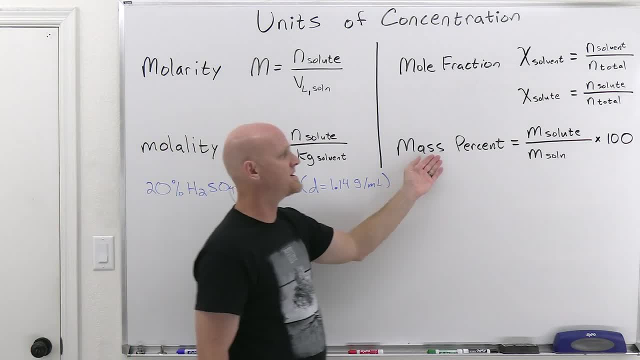 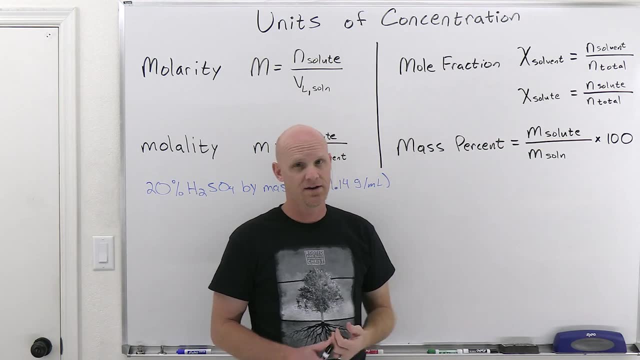 that way. And then, finally, mass percent. And so mass percent, in this case just a mass of the solute that you're looking at over the total mass of the solution times 100.. So, and again, you might have seen that before. What you might not have seen, though, would be like parts per. 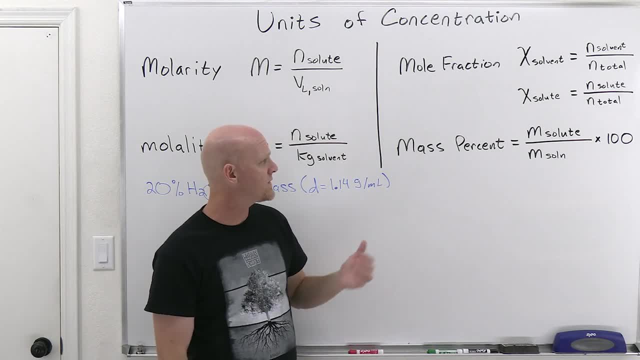 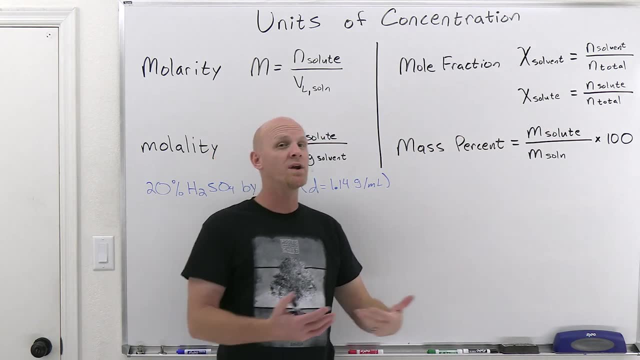 million or parts per billion or something along these lines. And what you need to realize is that a mass percent. percent means per 100. And a percent here is the same thing as a parts per 100.. And so you just take mass of solute over mass of solution times 100. 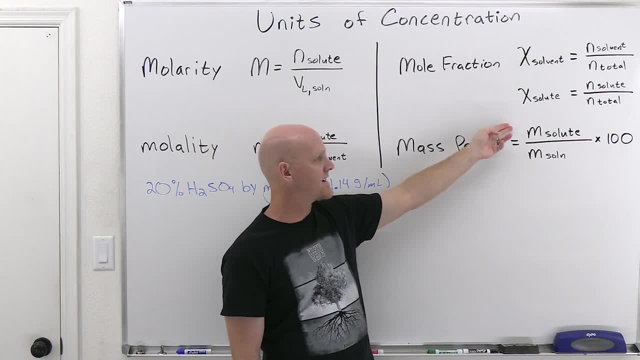 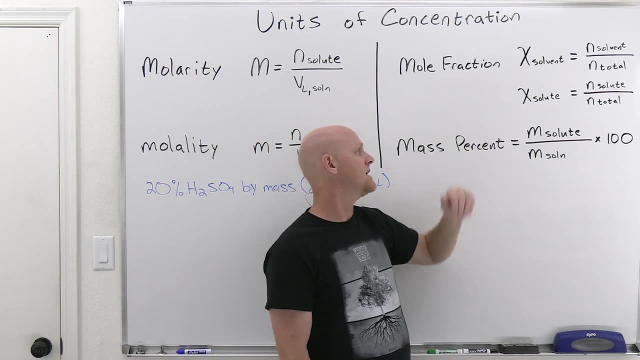 Well, if you're doing parts per million, you just do mass of solute over total mass of solution times a million, times 10 to the sixth. If you're doing parts per billion, it would be the same thing: Mass of solute over mass of solution times a billion. Now it turns out- we'll see that we 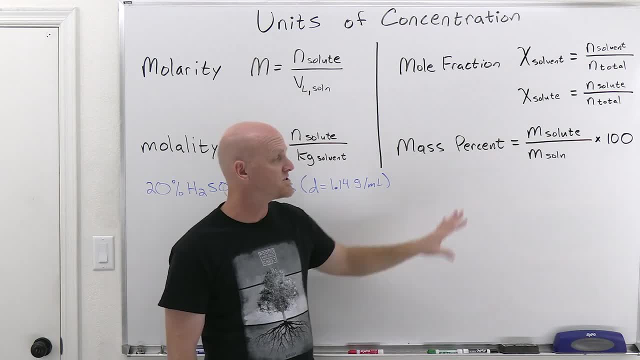 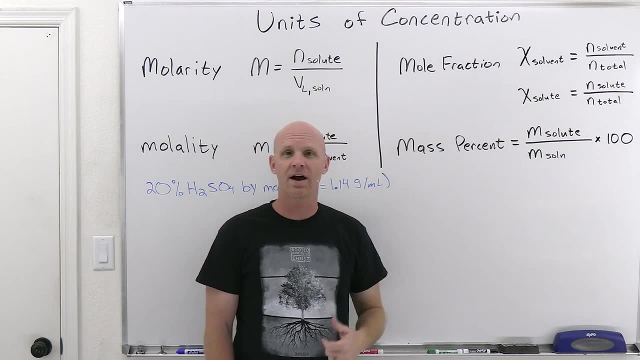 have some creative ways for aqueous solutions of not actually representing it that way and stuff like that. But you can always go right back to this Mass of solute over total mass times. the appropriate factor Again: percent times 100, parts per million times a million parts per billion. 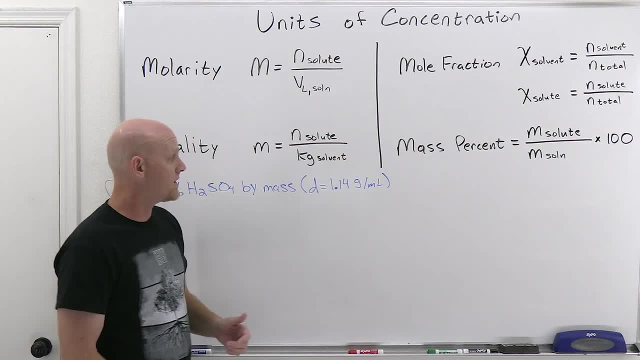 times 10 to the ninth, And so you can always go right back to this Mass of solute over total mass times a billion. Cool, So we're going to start with a 20% H2SO4 solution by mass, And we're 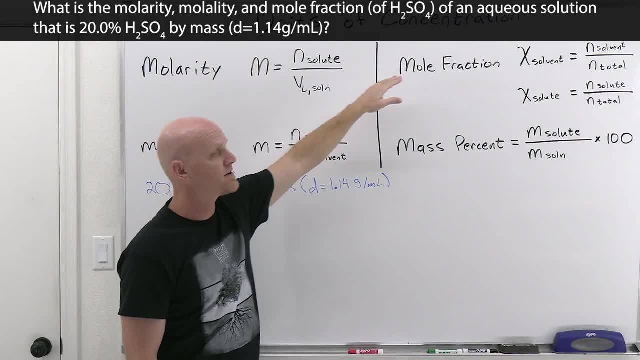 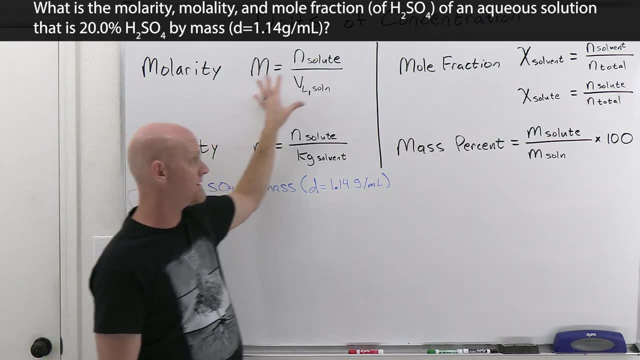 given a density here And we're going to convert it to each one of these other various forms of concentration and go from there. So you can kind of get an idea of how you would go about doing this. And again, you should be prepared for giving a concentration to any one of these four. 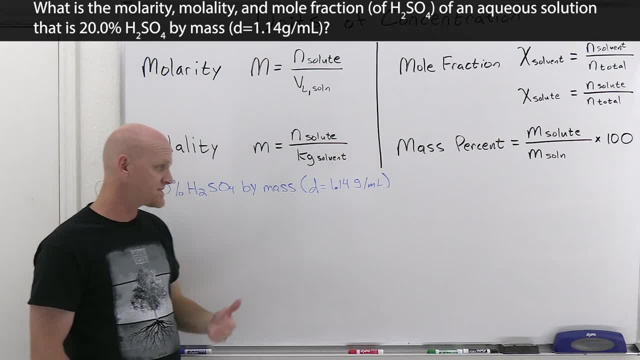 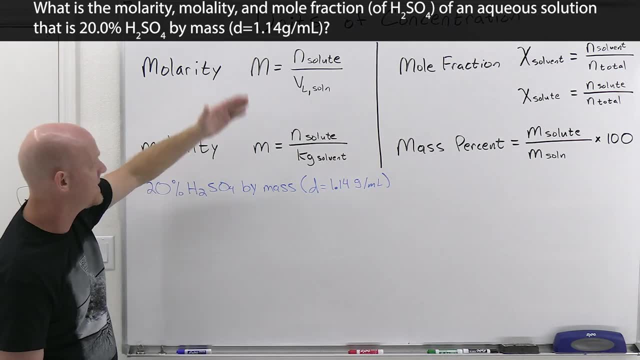 expressed in any one of these four and being asked for one of the other four. Well, in this case I'm giving you one of the four mass percent here and we're going to get all three of the others, And we'll definitely start with molarity here And so 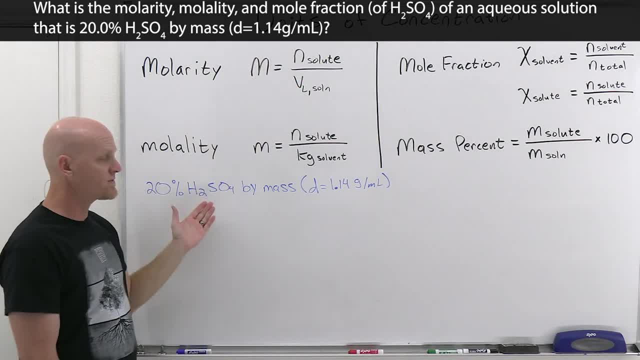 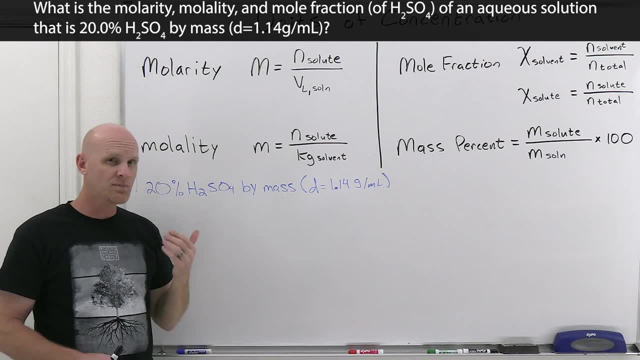 molarity is moles of solute over the total liters of solution, And so we've got to figure out how to come up with the moles of solute as well as the liters of solution. Now, one thing you're going to find helpful here is that these units of concentration, all of them, are intensive. 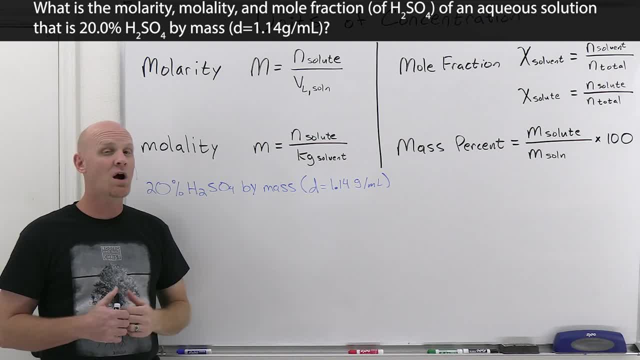 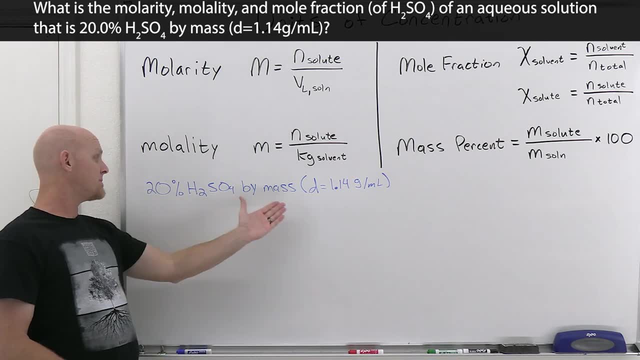 properties, And way back in chapter one, we learned that an intensive property is one that does not depend on sample size whatsoever, And so in this case, we don't have a sample size. We're just told that we have some variable amount of this 20% H2SO4 solution. We're given its density. 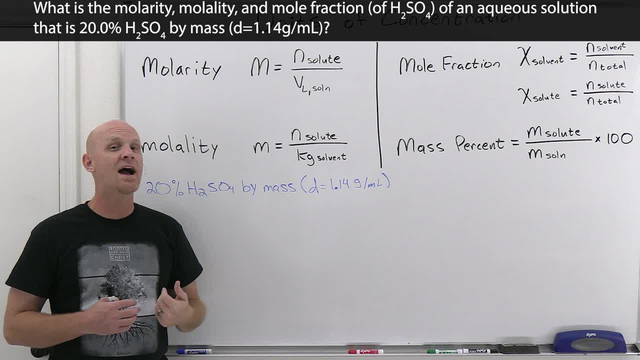 but we don't actually have a sample size. So we're just told that we have some variable amount of this 20% H2SO4 solution, And we don't actually know how much we have, And so in that case you can. 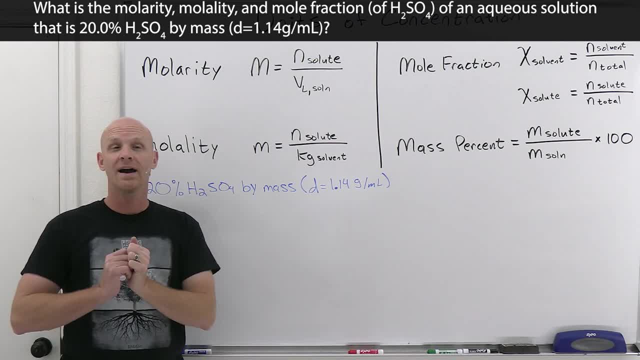 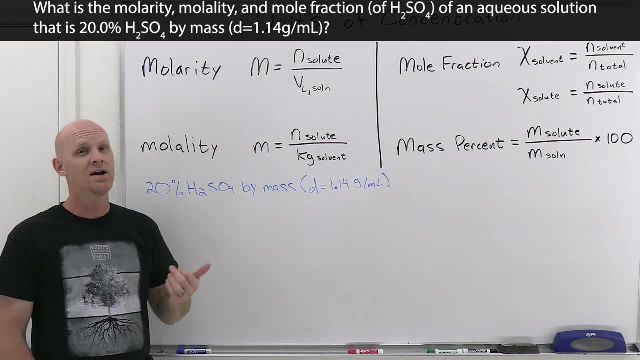 actually choose how much you have. It is up to you, And it doesn't matter what you choose. You're going to get the same answer for the other forms of concentration here, regardless of what volume you use. Now you might choose a rather convenient volume to make your life just a little bit easier. 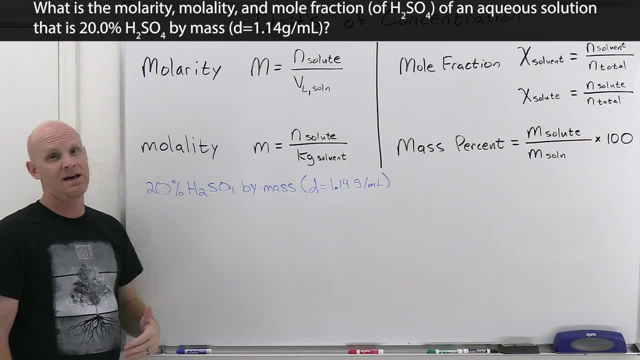 And so, in this case, being given like a percent mass, it might be really convenient to choose a 100 gram sample size, And the reason we might want to do that is because, well, 20% of 100 grams we can do in our head, And so we're going to have a sample size of 100 grams, And so we're going to 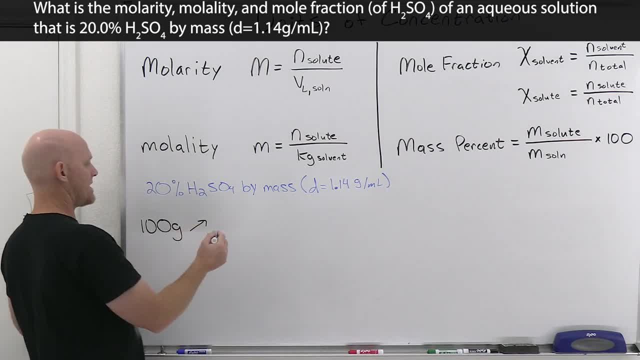 be 20 grams of H2SO4.. And again, our goal here is to take what we're given here and get the moles of solute and the total volume in liters of the solution. So we can start with this: 20 grams of. 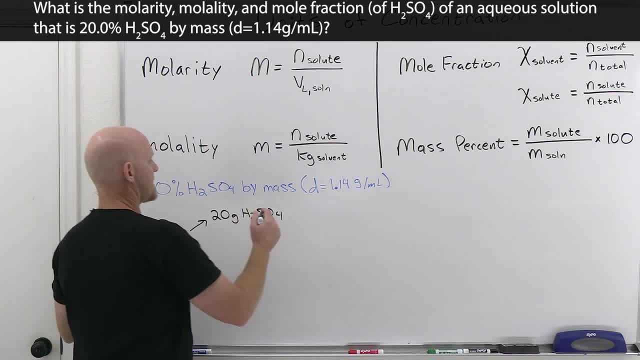 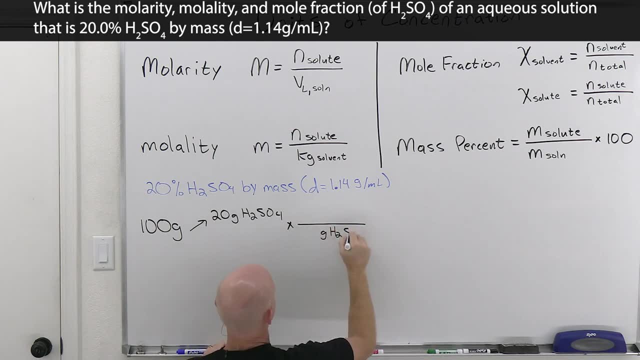 H2SO4, and we can turn that into moles, And so that'll be our first step here, And to get from grams to moles, we just use our molar mass here, And so we're going to take that grams of H2SO4,. 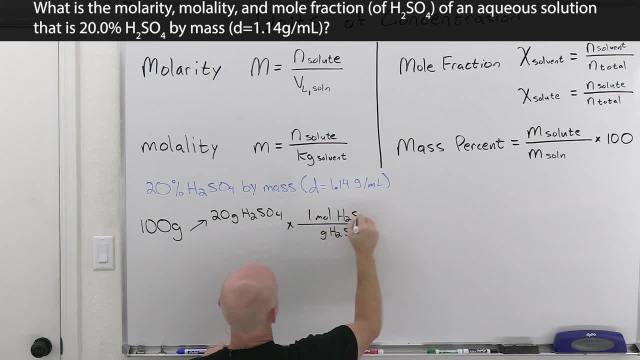 that are in one mole of H2SO4. In this case, two hydrons is two, sulfur is 32, four auctions are 16 inches, a total of 64.. 64 plus 32 is 96, plus two is 98 grams per mole, And so we'll do 20 divided. 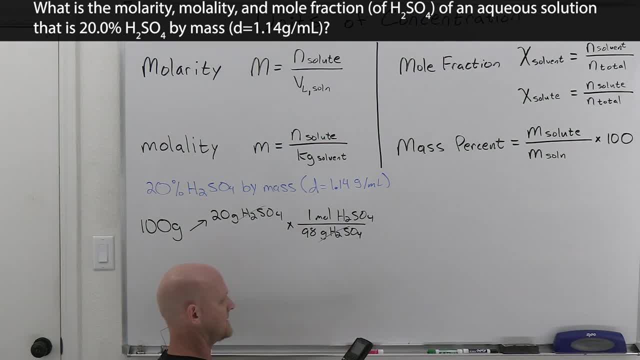 by 98 here and pull out the calculator, 20 divided by 98 should be roughly one fifth and it's 0.204.. Cool, And that's our moles of H2SO4.. Cool, Now we got to get the total volume again in liters of. 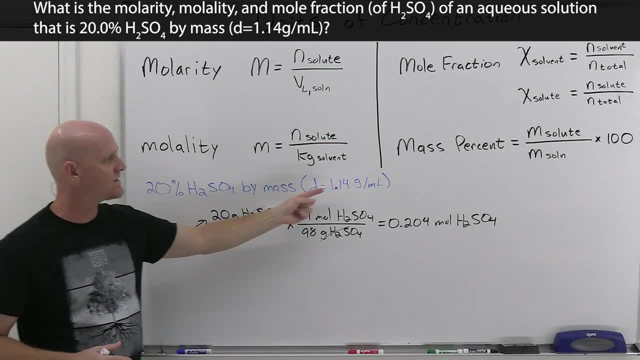 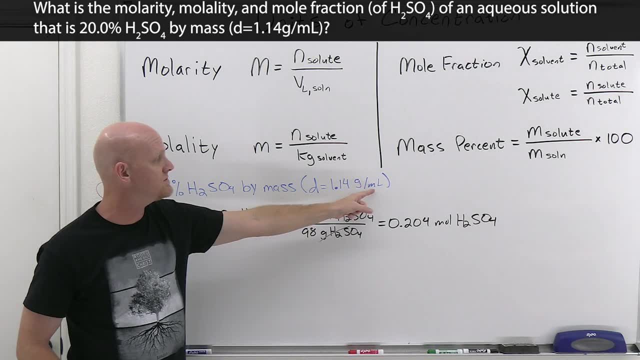 the solution, And in this case, that's what our density is for. Our density relates the mass to the volume. Well, we know the density, We've chosen a convenient mass, the 100 grams, and we can now use that to get that volume. And so here you've got to remember that density equals mass. 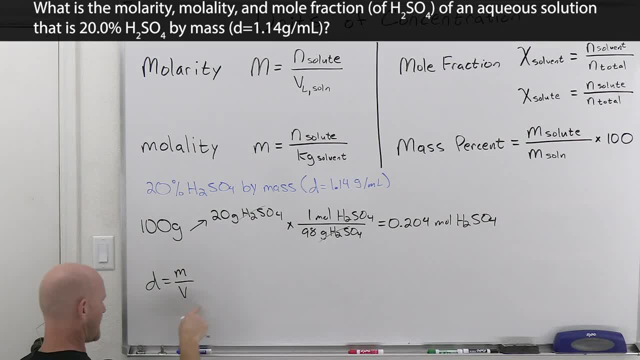 over volume, And if you arrange this, you could bring volume up over here and then divide through by density, And so we've got to get the total volume again in liters of the solution, And so you find out that volume equals mass over density, And that's what we're going to use here. So in our 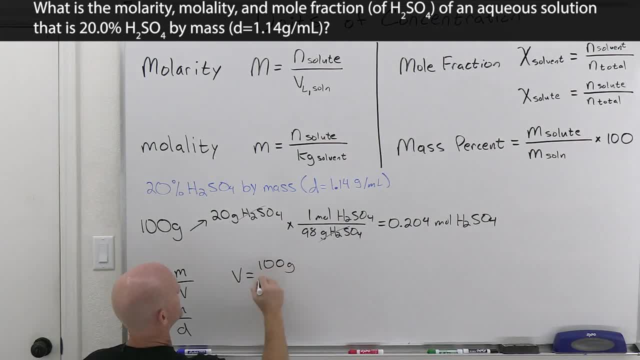 case we know the mass is 100 grams, We chose that The density was given as 1.14 grams per milliliter And in this case this is going to come out in milliliters, So we could convert it. 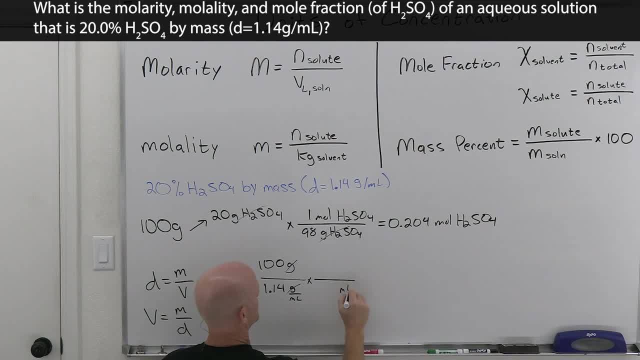 after the fact, or just do it right here And we can turn milliliters into liters, And one liter is 10 to the third milliliters. Or you could have said: one milliliter is 10 to the negative three liters, which is 10 to the third milliliters. So we could have said one milliliter is 10 to the. 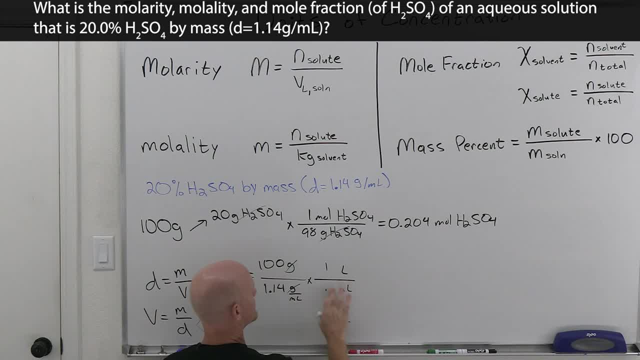 three liters, which is technically my preferred way of doing it, But most of you probably do it that other way there. So but one milliliter is 10 to the negative three liters. That way the one goes in front of the unit with the prefix and the unit without the prefix gets the power of. 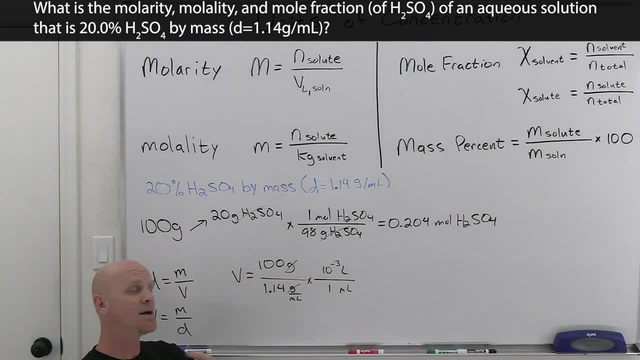 10.. So again, just want to make sure you realize why I'm doing this, maybe in a way that maybe is not the most normal, typical way. you're doing this So, but in this case we're ready to pull out that calculator again And we're going to do 100 divided by 1.14, and then times. 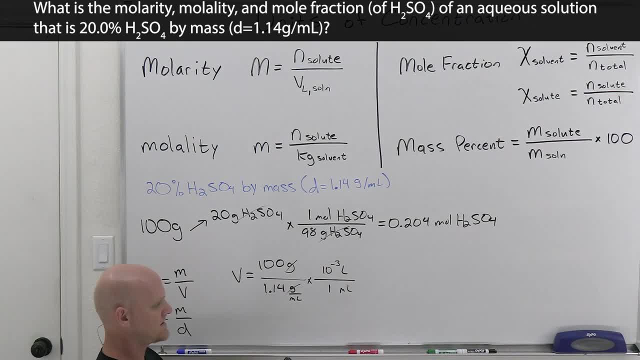 10 to the negative three, and we're going to get point 0877 liters. And now we're ready to go. we've got the moles of solute, we've got the total liters of solution, we're ready divide one by the other to get our molarity here. And so in this case, 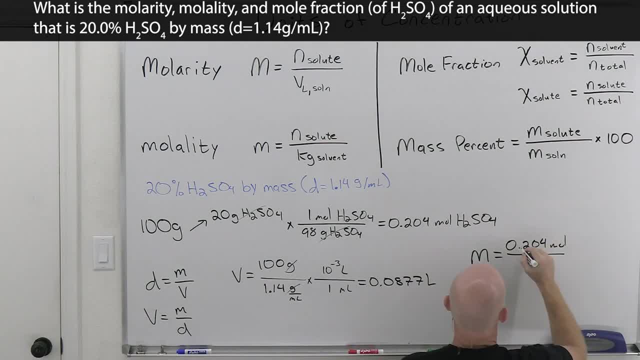 we're going to have that 0.204 moles over a total volume of 0.0877 liters, And we'll see what our calculator tells us here. So 0.204 divided by 0.0877, 2.33 molar. 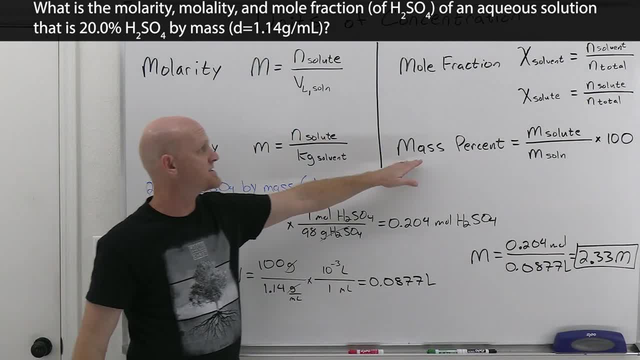 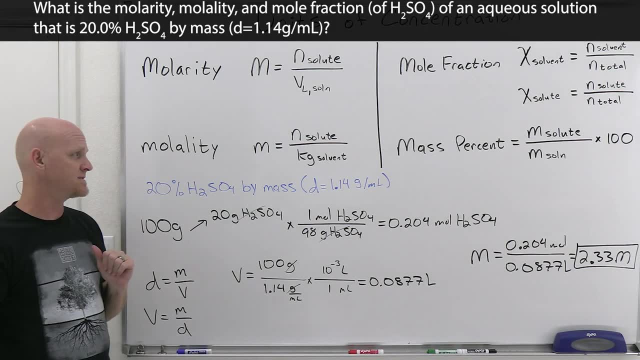 Cool, And that is step one. So now we took our mass percent and we used it to find the molarity. And again, it was convenient to remember that it's an intensive property and we got to choose the sample size. Cool Next up on the docket here is going to be finding now the molarity. 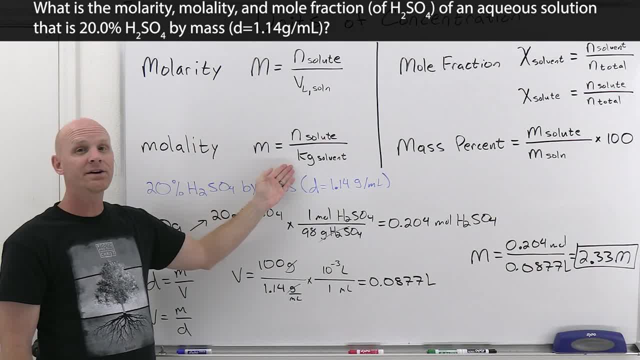 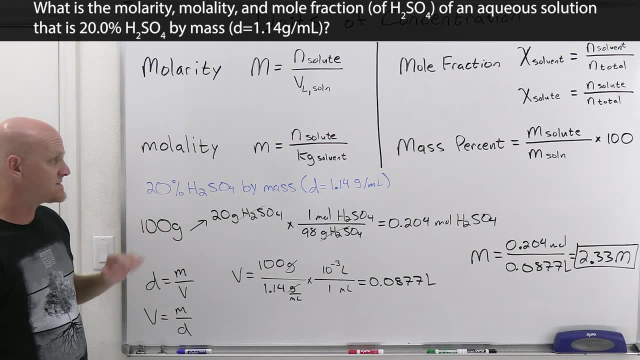 molality, And so in this case we want moles of solute and kilograms of solvent, And we could take the work we've already done here and kind of just do a little backtracking here. So in this case again, we can choose any sample size and 100 grams still becomes. 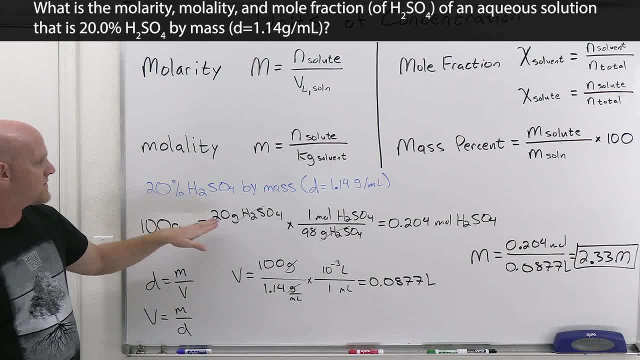 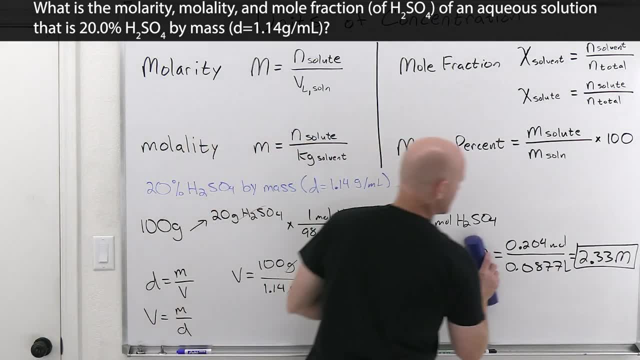 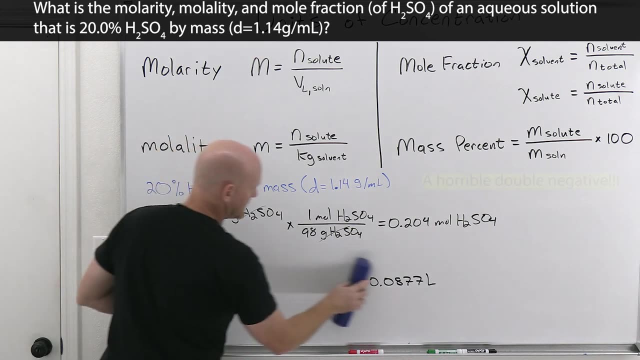 a convenient one in dealing with a 20% solution. So we still got 20 grams of H2SO4, and that's going to be helpful, And let's go backward here. So done with this, We're done with no, we're going to need that still. So, but the volume we don't need, no longer. So. but 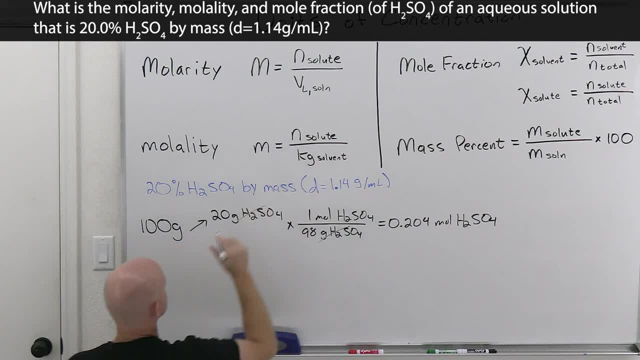 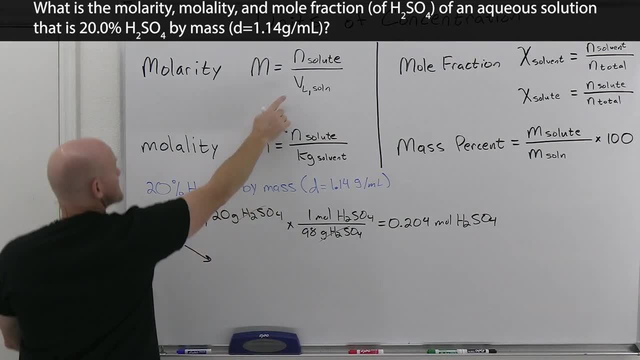 what we can figure out, though, is we need to know something about the kilograms of solvent. Well, in this case, we had 100 grams of solution, 20 grams of solute- What we never figured out before because it wasn't relevant, because we were talking about the entire solution. 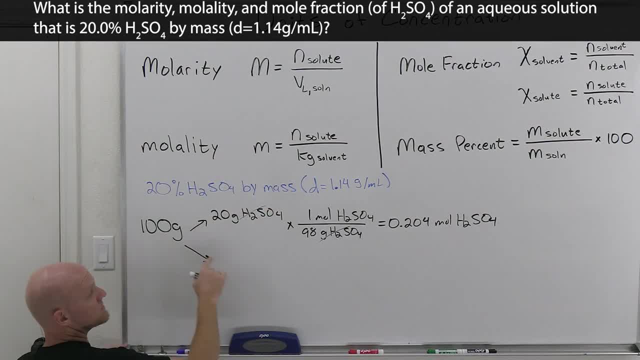 but now we just need the solvent. So if 20 of the 100 grams are solute, then 80 of those grams are going to be the solvent, And in this case It's water. but we just need to turn that grams into kilograms. 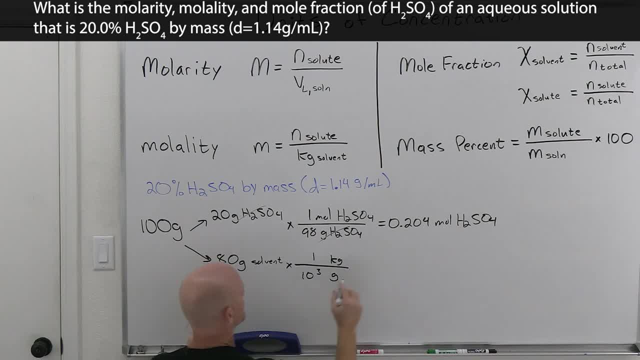 So, and in this case one kilogram is 10 to the third, or a thousand grams, and we'll get this. just divide through back three decimal places- 0.080 kilograms- and we're now ready to calculate out the molality instead, And so in this case it's 0.204 moles over 0.8. 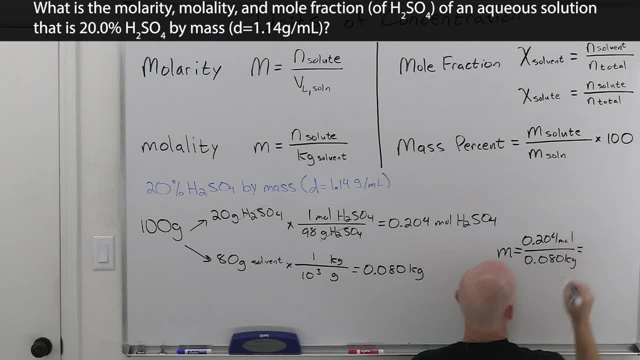 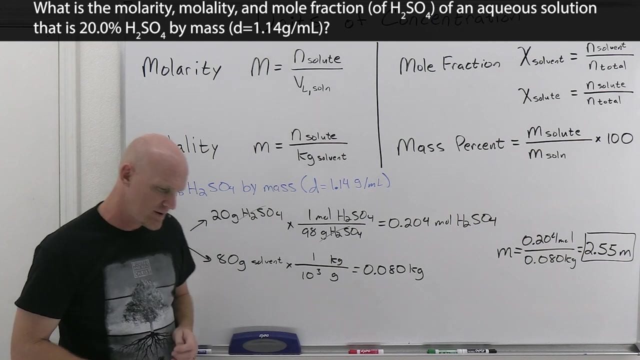 milligrams, And we're going to get 2.55 molal, the way we say it, Cool. And so here we see that the molality is just a little bit higher than the molarity we had previously calculated. One thing to note here again is that, as we add, solute, the total volume of the solution. 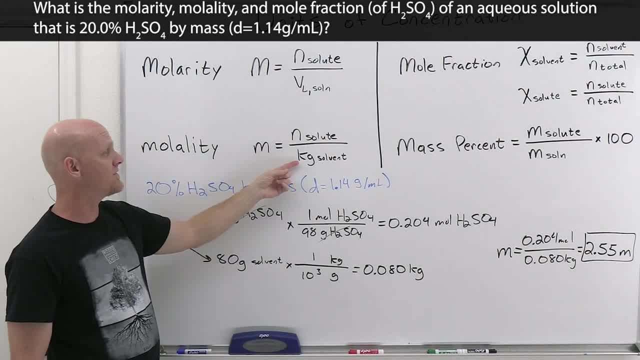 will in all likelihood for most solutions increase. there's usually an expansion there, But again, the kilograms of solvent does not change. What's interesting is that, as long as you're dealing with an aqueous solution where you've got water, one kilogram of water is one liter of water, roughly depending on the temperature. 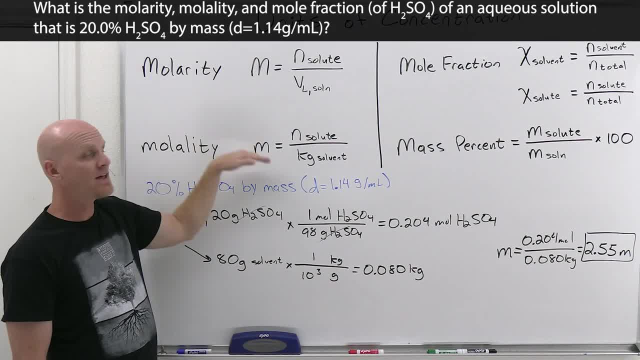 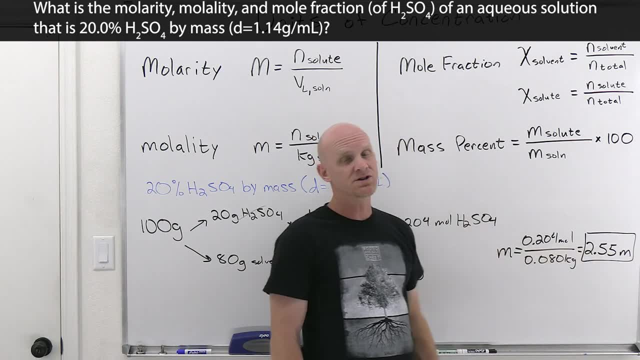 And so for fairly dilute solutions, the molarity and the molality are actually rather close to each other. But as you get a more and more concentrated solution, you'll see a bigger and bigger deviation, usually with a higher molality, just as we've done here. then you do have a molarity. 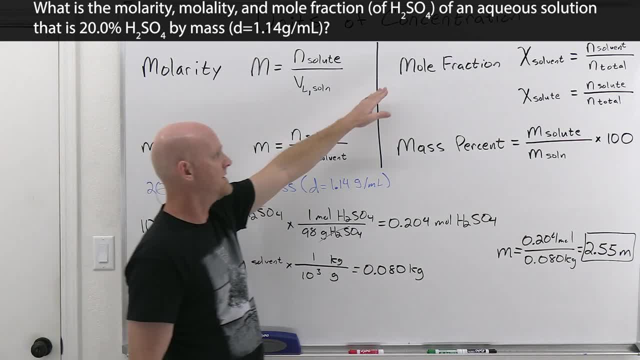 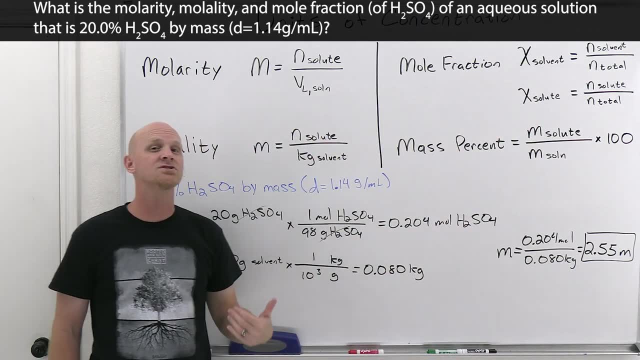 Okay. so last one here. we've got to find mole fraction, And in this case they've got to tell us which mole fraction they want. Do they want the mole fraction of the solvent or the solute? Well, in this case, I want the mole fraction of the solute. 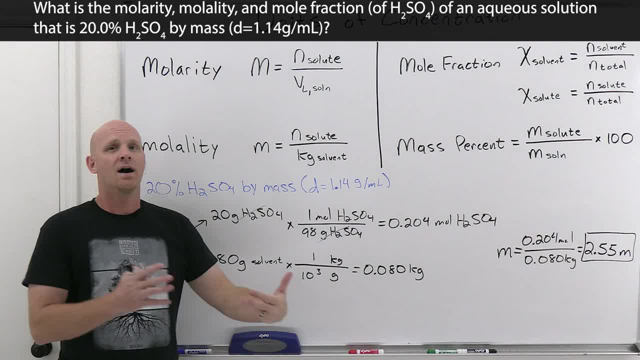 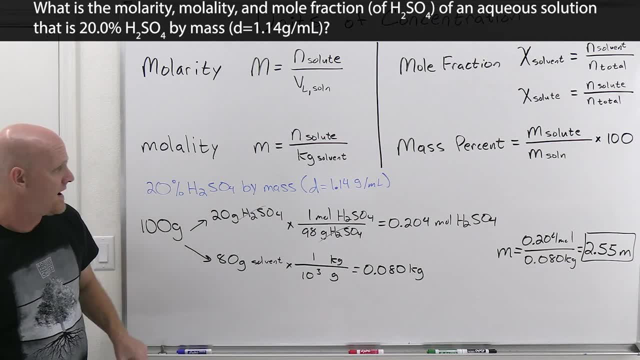 But we'll find out with one of our colligative properties. in the next lesson that actually is going to be, you're going to be needing to know the mole fraction of the solvent in such a case as that. So we're going to deal with this mole fraction of the solute. 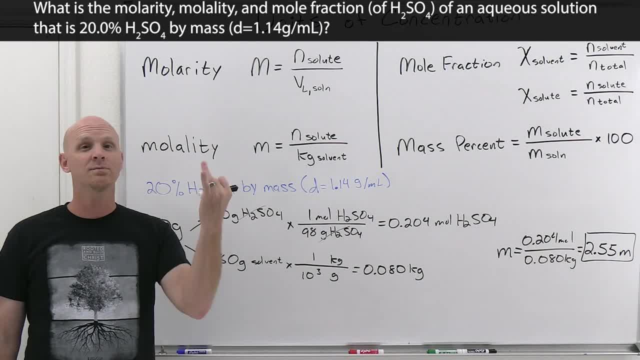 And to get the mole fraction of the solute, I need to know what the moles of solute and the moles of solvent, both In this case. we know the moles of solute. that's something we've already calculated. 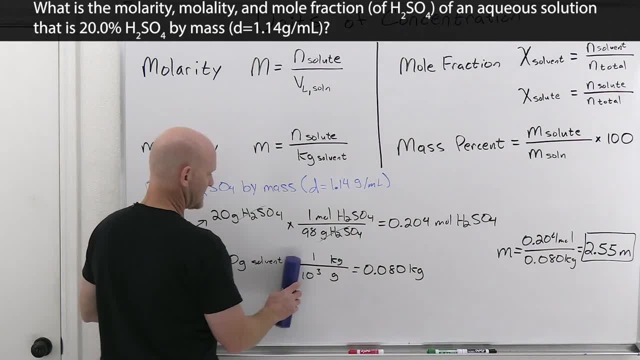 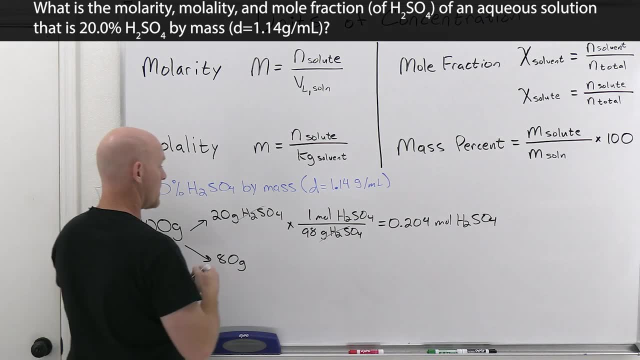 here with this 0.204.. So we're going to keep that. So we're going to take that 80 grams of solvent here in this case, and instead of just calling it solvent, we'll call it water, say aqueous solution. 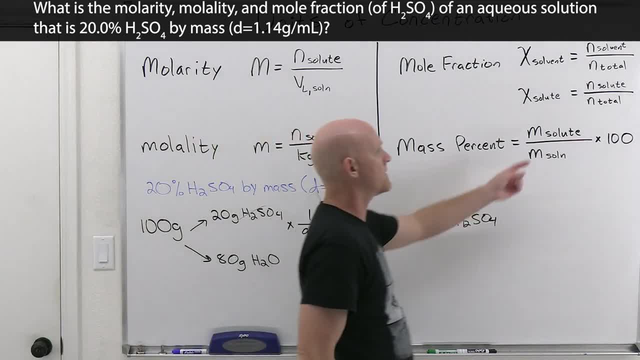 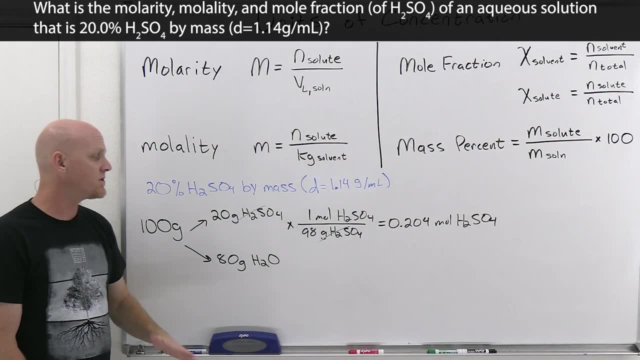 So instead of converting it to kilograms now, I need to convert it into moles. So this total moles in this point here, total moles is both solute and solvent combined, And so again, we've already got the solute, but I need the moles of solute. I'm sorry. 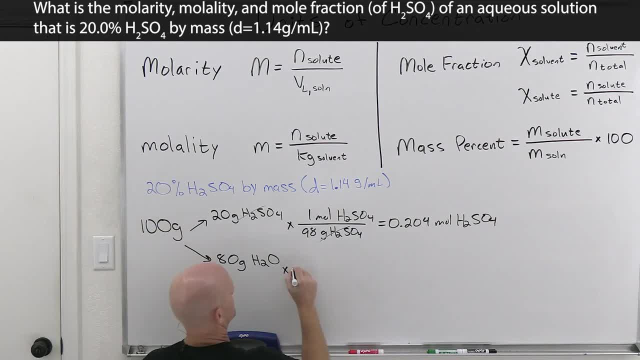 moles of solvent in this case, And again our molar mass right off the periodic table for water oxygen: 16, the hydrons are each one, So a total of 18 grams per mole, And 80 divided by 18 is 4.44. 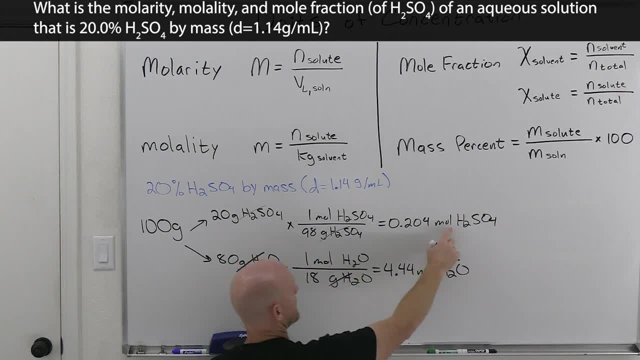 Okay, so we want that mole fraction for H2SO4. here We'll take the mole fraction for H2SO4.. We're going to get the moles of H2SO4 all over the total moles, which would be a combination. 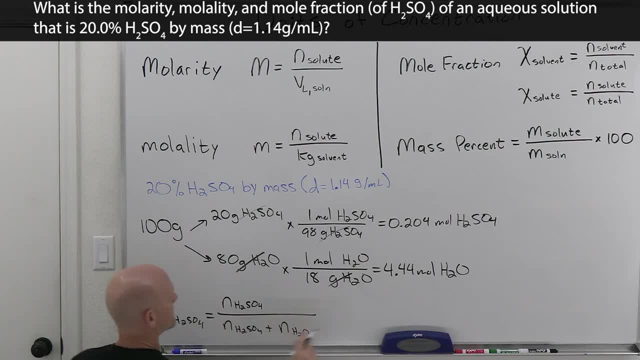 of the H2SO4 and the water, And so in this case we'll have the 0.204 all over 0.204 plus 16.. Okay, Okay, Plus 4.44 to get our mole fraction. All right. 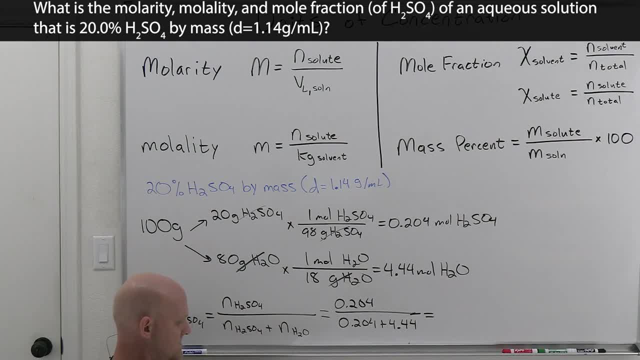 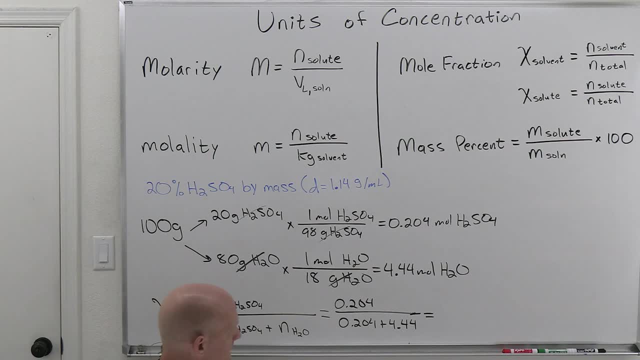 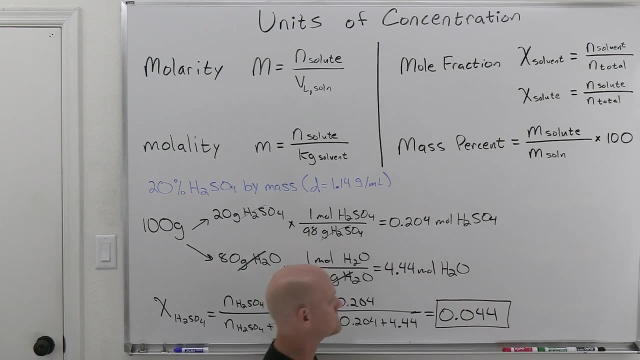 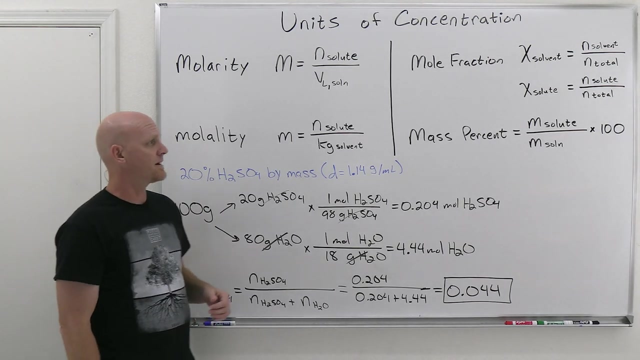 So 0.204 divided by parentheses, 0.204 plus 4.44 in parentheses, and we're going to get a mole fraction of 0.044.. Cool, And again, we've now done every conversion you needed. And again, real quickly, we started with mass percent. 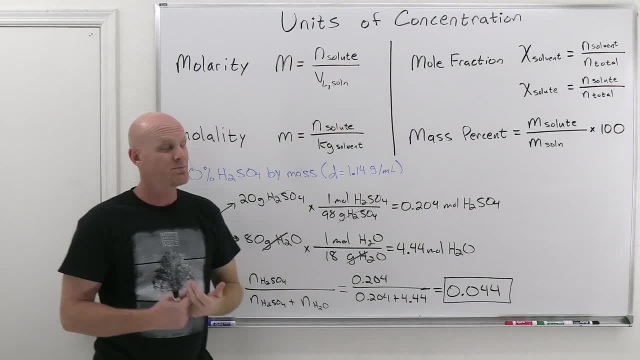 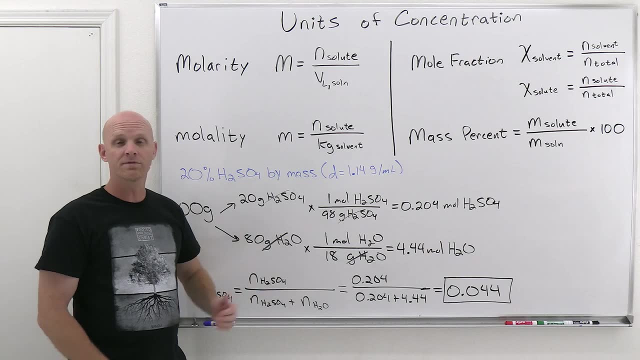 We found the molarity, then the molality, then the mole fraction And, in principle again, you could have started with any one of these and been asked for any of the others, And I just wanted you to have an example where you've seen it performed for all of them. 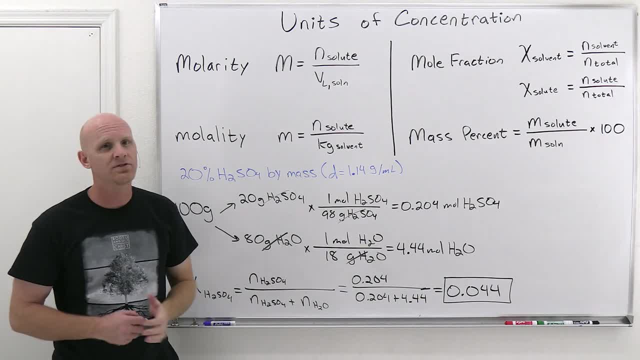 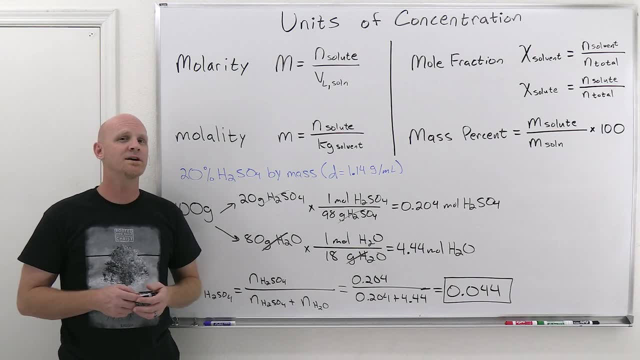 And once again, we're going to use both molality and mole fraction in the next lesson on colligative properties. So, real, convenient. We've reviewed them here Now. if you found this lesson helpful, thumbs up goes a long ways to making sure YouTube. 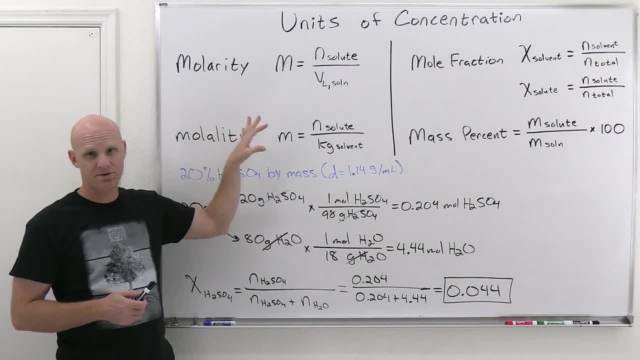 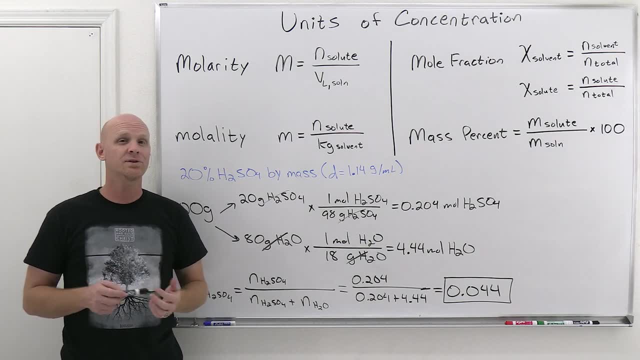 shares this lesson with other students. And if you are looking for practice materials for your gen chem course, my general chemistry master course includes over 1200 practice questions, And if you're studying for finals, it also includes final exam rapid reviews, where I 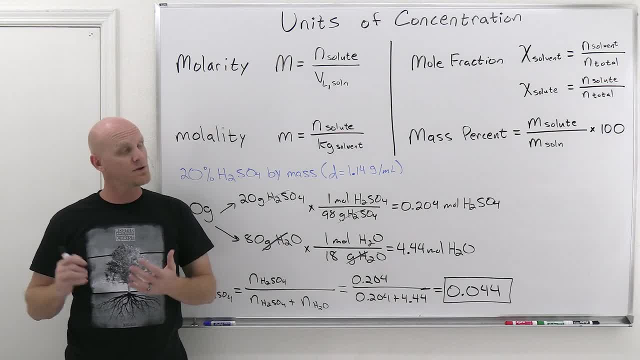 review all of the topics in gen chem one in roughly five to six hours, or all of the topics in gen chem two, also in roughly five to six hours. also includes practice final exams. You can find a link in the description of free trials available. Happy studying. 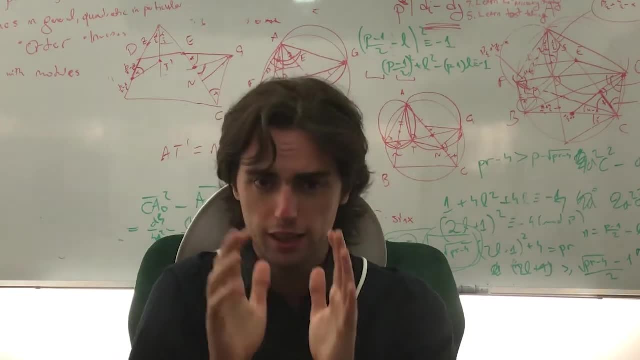 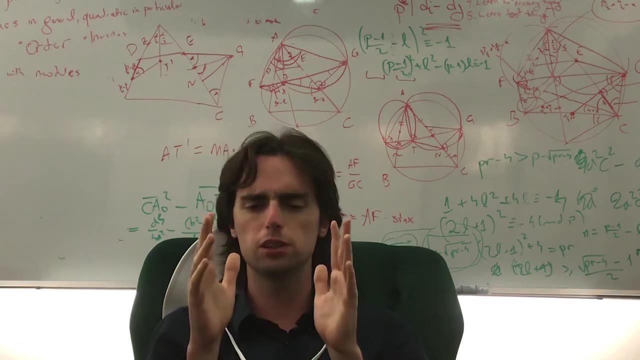 Hello, fellow problem solvers. So today we're going to be talking about invariance and I've made a video on and I've sold a couple of problems with invariance. but now I want to focus just on the general concept overall. What is it? How do you do it? 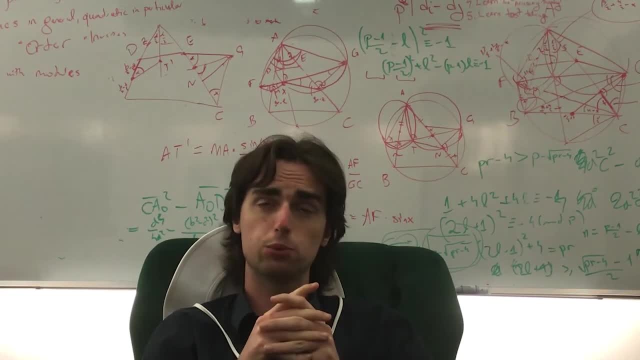 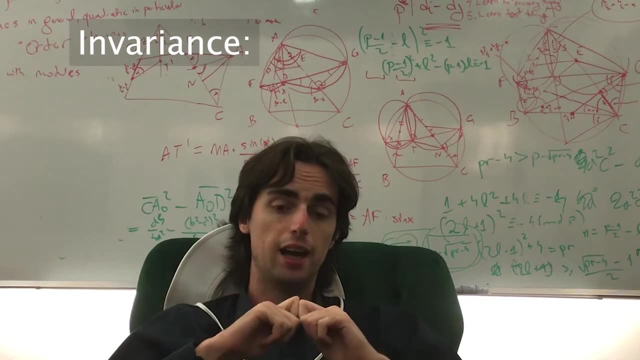 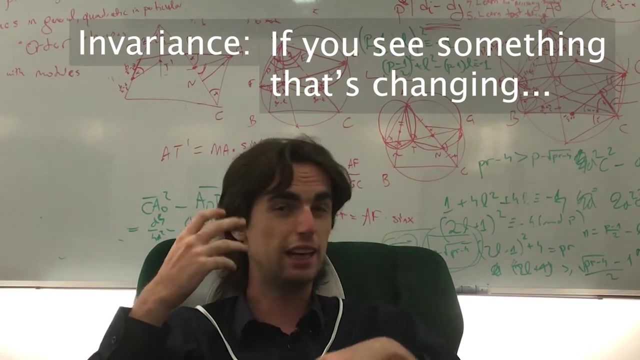 And the first really step is: what is invariance? It's really a higher order problem solving technique. It's saying that when you're working on a problem and you see there's something that's changing in the problem, Say there's some transformation that's happening. again and again. 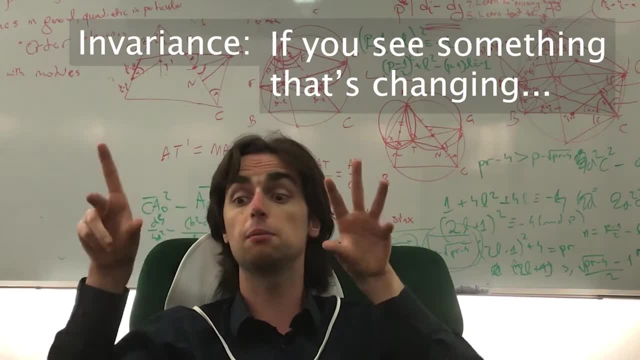 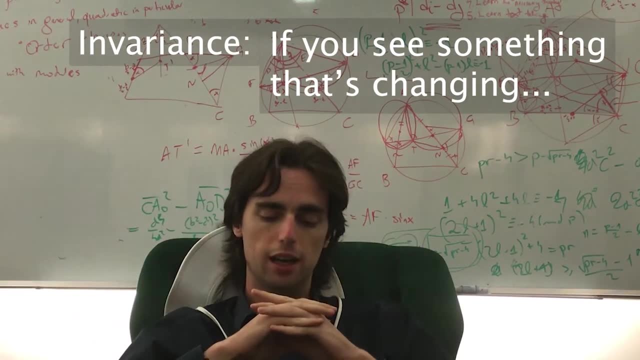 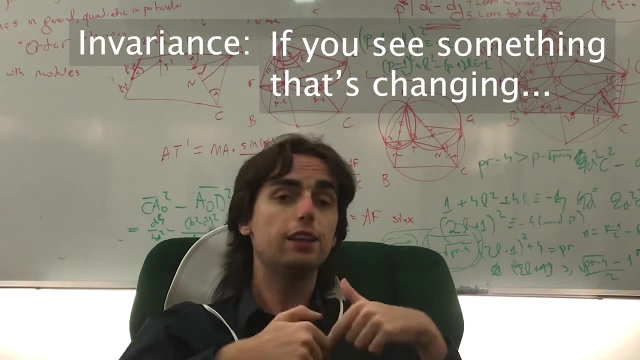 It might be happening differently at different times, but there might be something that's the same as it's happening. You might see this in games or whatever, and or any sort of like algorithmic changes that are happening. You ask yourself, while this change is happening. 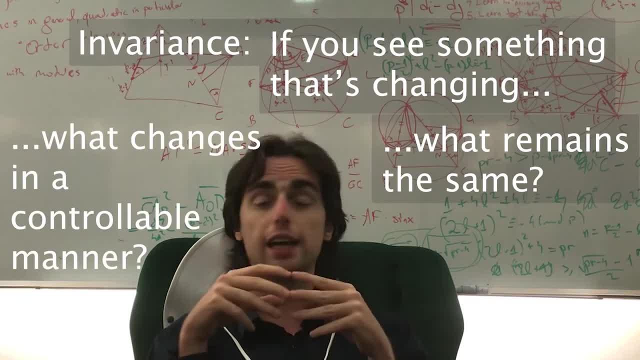 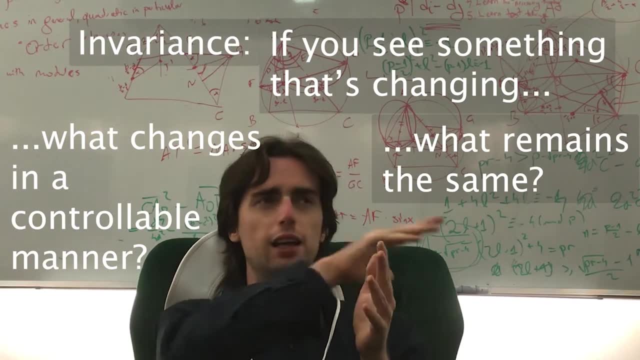 what is something that remains constant, or something that remains constant, What is something I can really control, And when I say control, what I really mean is something that you can model or evaluate algebraically, evaluate like a value of something and say a good. 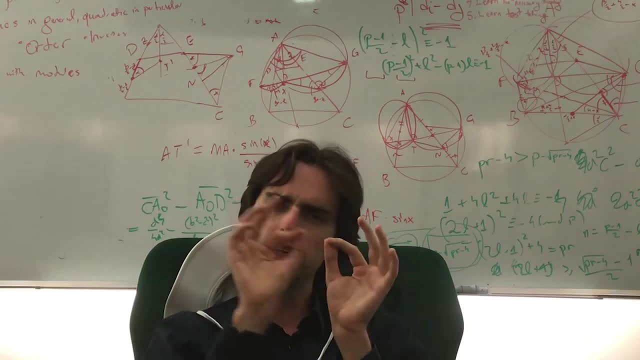 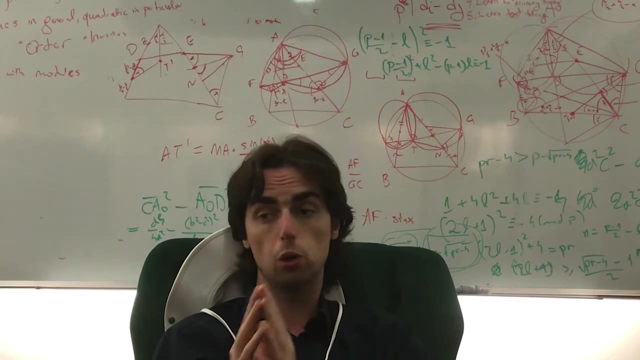 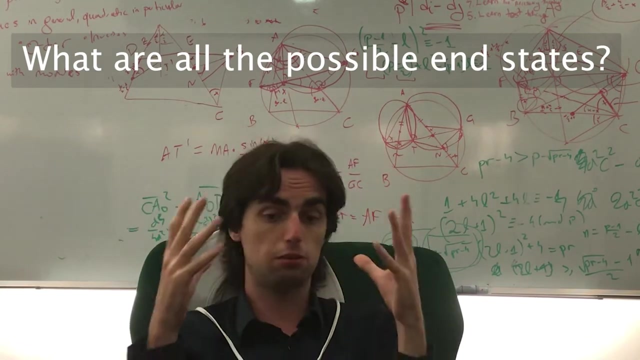 example of invariance. Actually, before we get into the example like, here's a couple of questions that you can ask yourself while you're seeing these changes happening in problems. One of them is: what are all the possible end states? So a state of like? there's a state that the problem is in.